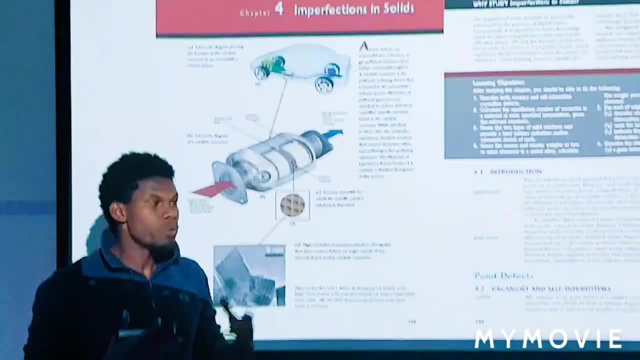 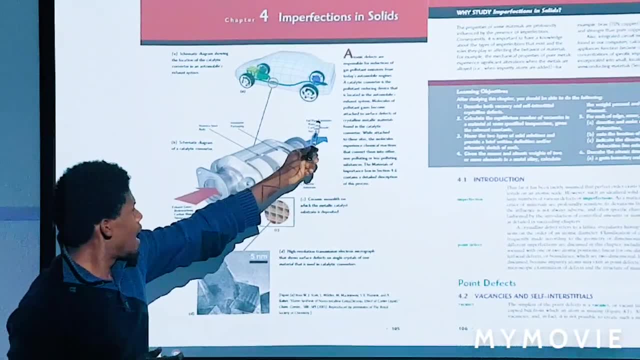 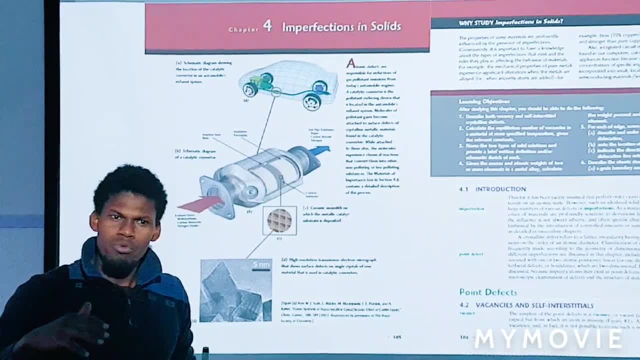 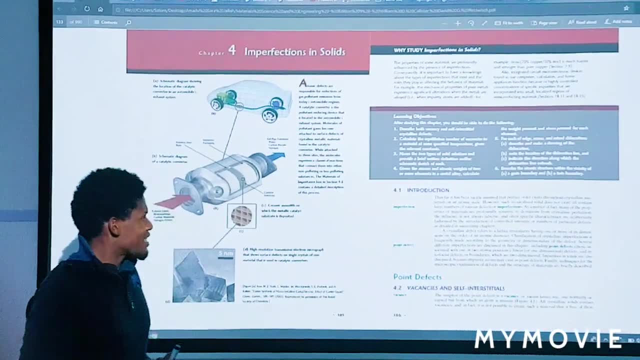 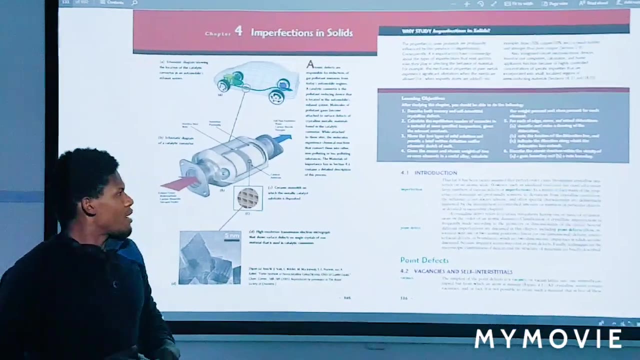 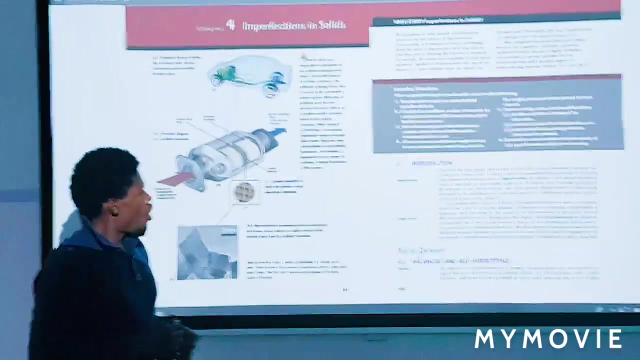 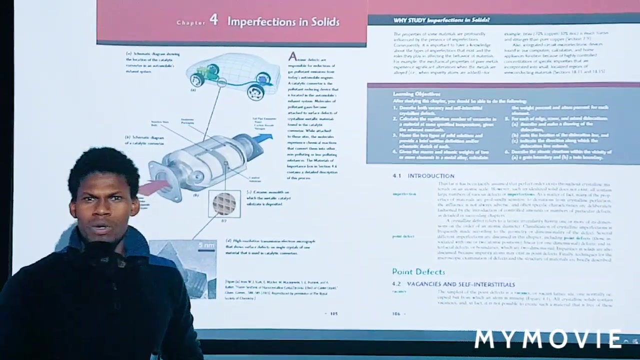 And upon this process they are undergoing some chemical reactions. computers in our household, machines, everywhere. If we understand, right from the atomic level, the importance of understanding imperfections in solid materials, then we can be able to design materials to meet our daily needs. We can be able to control these materials. 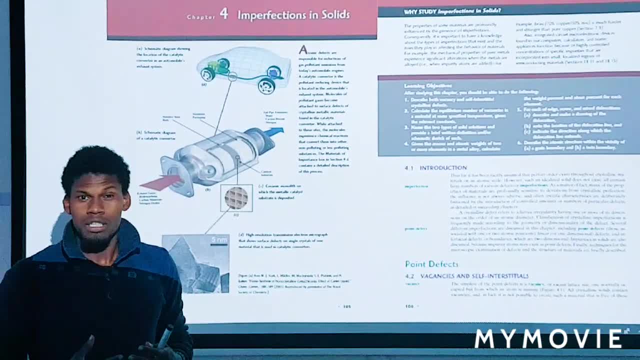 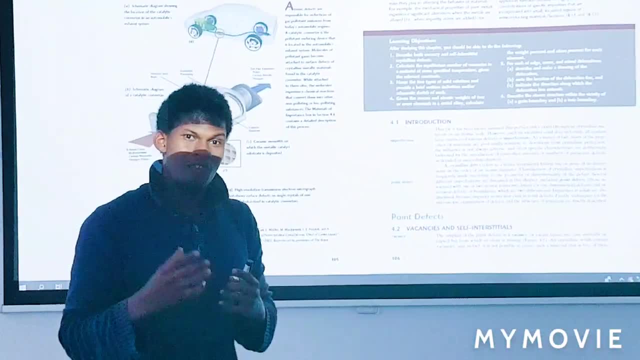 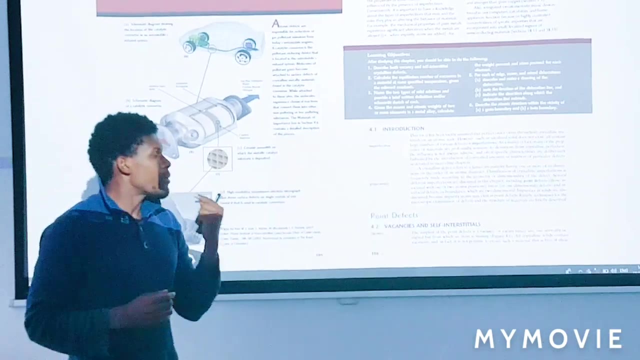 So that's why we should study imperfections in solids, And these dictate the properties of materials. And we know that, whatever that dictates the properties of materials, you should know that you should be able to study these properties, these structures and how these materials are performed. And the only way we can be able to manipulate this is for 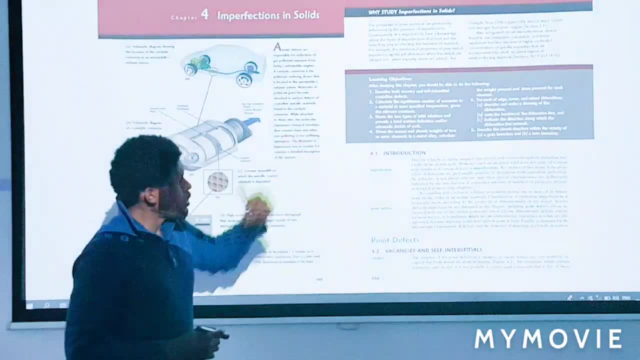 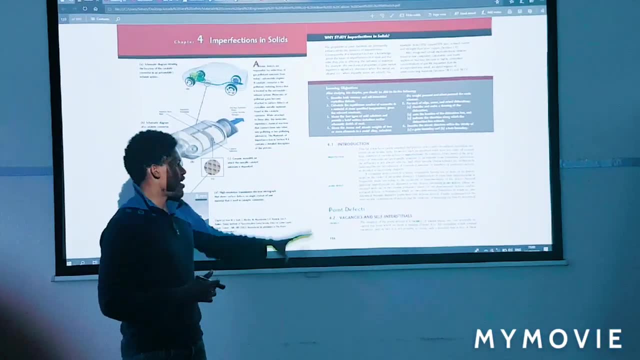 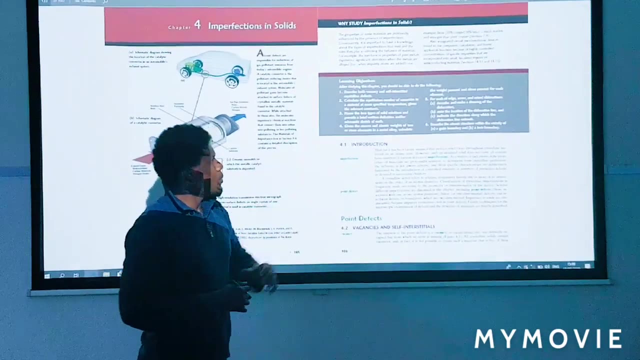 us to be able to study these things. So here is our learning objective. What are our takeaways? What can you take home with you when you study material science and engineering, and especially chapter 4, imperfections in solids? So, number one, you should be able to describe what vacancies. and set of decisions are. And number two: you should be able to describe what vacancies and set of decisions are. And number three: you should be able to describe what vacancies are. And number four: you should be able to describe what vacancies and set of decisions are. 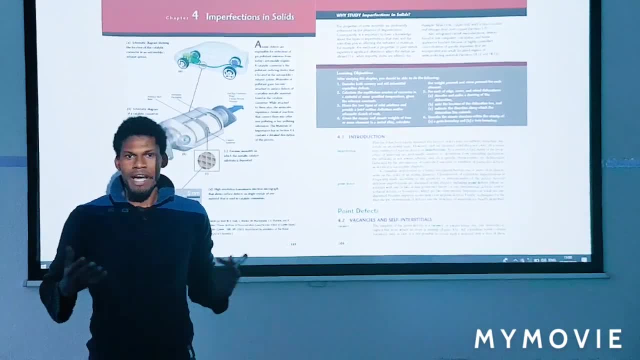 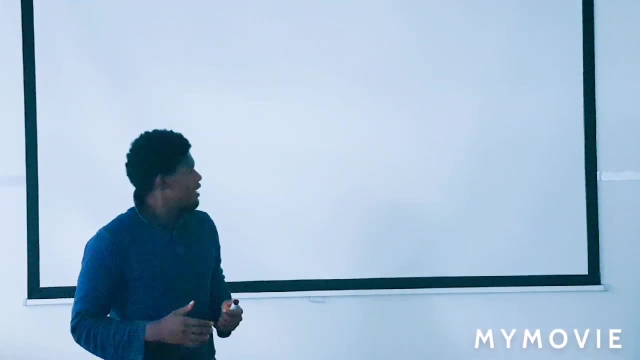 I know most of you are familiar with what vacancy is right When you are looking for a job, for example. you go out there and you search for a job, you get a job And upon this job, when you are looking for a job, you have vacancies All right, all along. we. 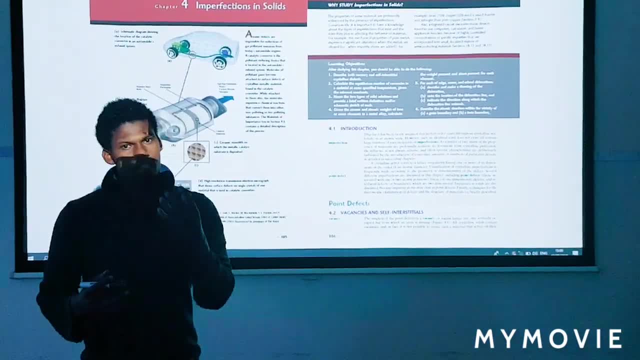 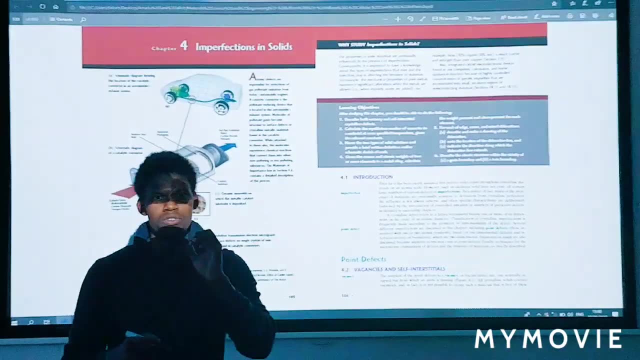 talk about chapter 3, as we know, about polycrystalline materials and single crystal materials, And we say that materials are perfect. But this is wrong. There is no material that is perfect that doesn't have some vacancies. So we're going to talk about polycrystalline materials. 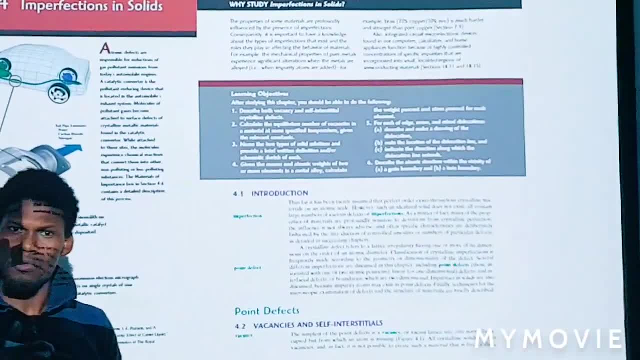 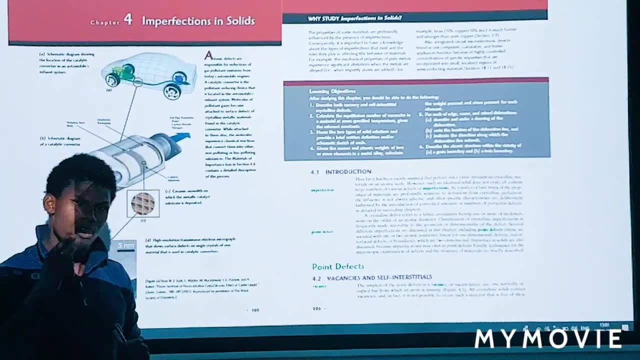 to see vacancies and separate interstitials and we should be able to calculate how many vacancies are present in every material. how many defects are in India. so you should be able to know that and you should be able to calculate these things, because only then you can able to control how. 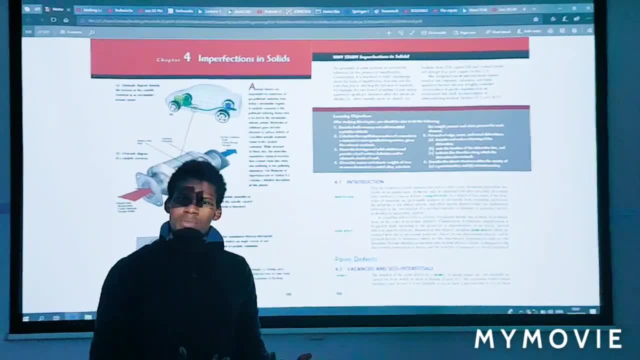 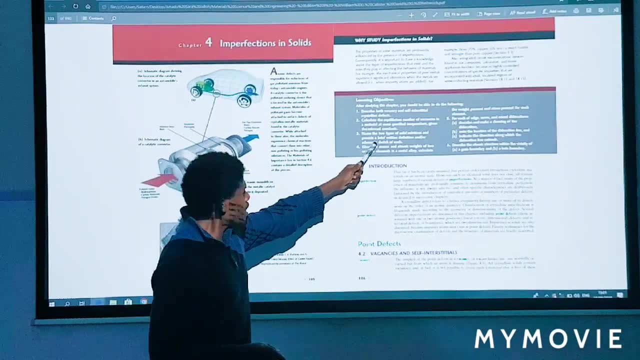 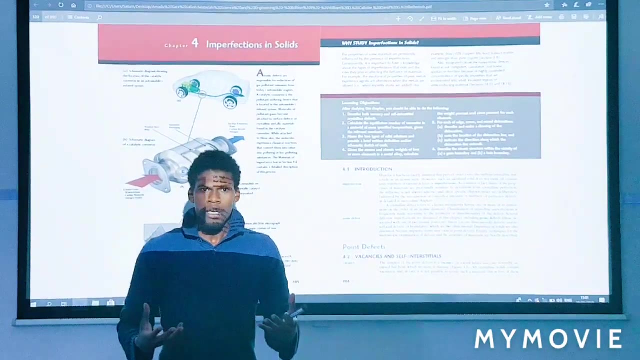 these things, how these vacancies affect the properties of these materials. so you should be able to. that's the takeaway we're going to take with us at home after we finish studying this course. another thing is the solid solution substitutions we have like, for example, a simple analogy with with water. if you are mixing water with alcohol, you cannot able to differentiate it. 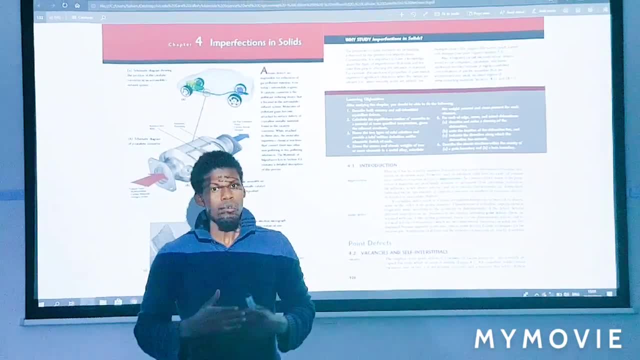 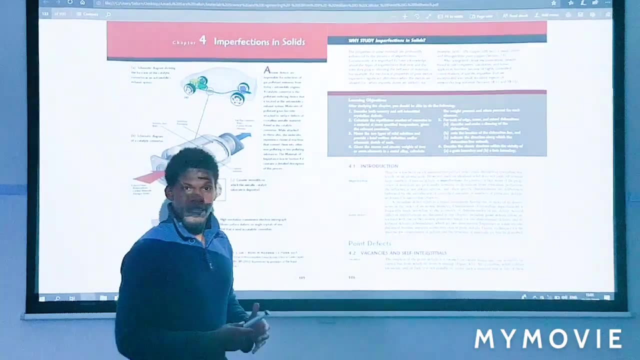 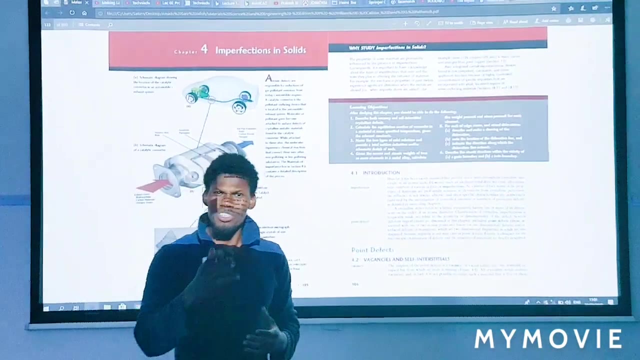 until you test it, then you know that, yes, there is mixture, so it's the same to it. solid materials: we can mix two solid materials. we can mix copper and zinc to determine that, and another thing will be the masses. how can you calculate these masses? because it's very important. so, for example, if we mix copper and zinc, you want to know how much of 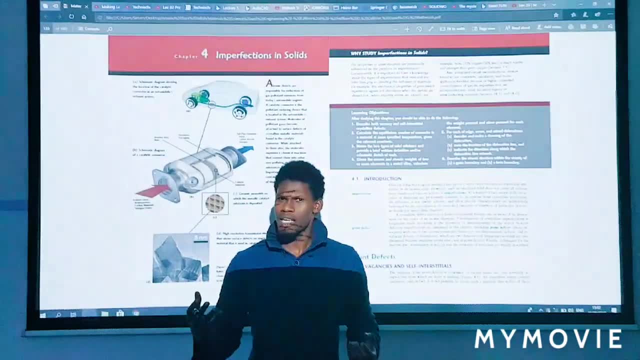 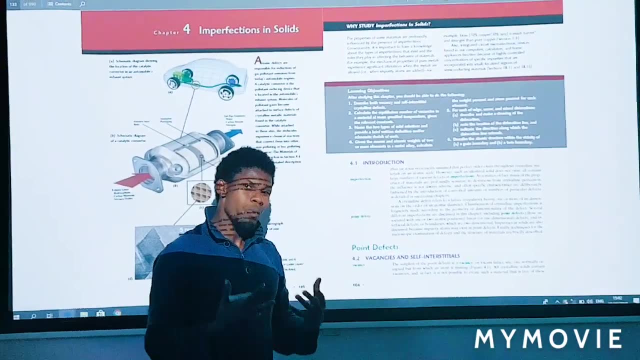 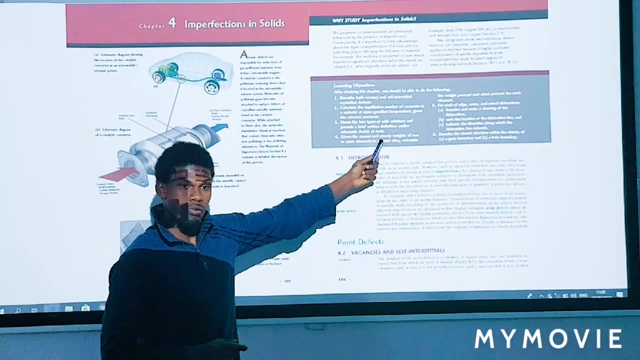 copper do you have within this material, and how much of zinc? because when you combine these two you have alloyed material. so you should able to determine the weight or you should able to determine the number of atoms that are within this material. so that's the take away we should. 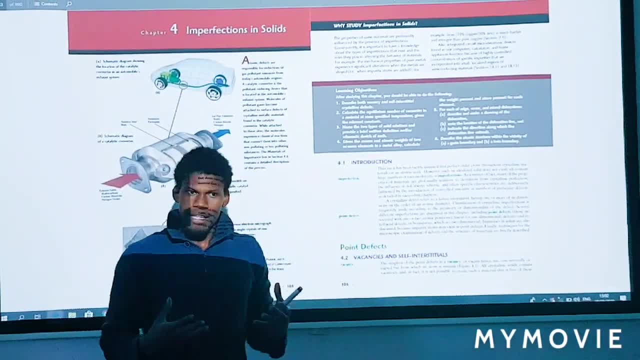 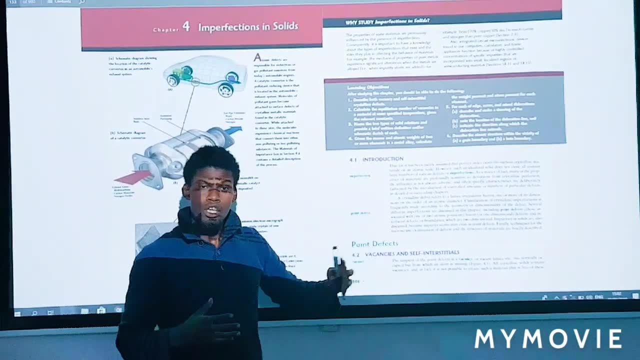 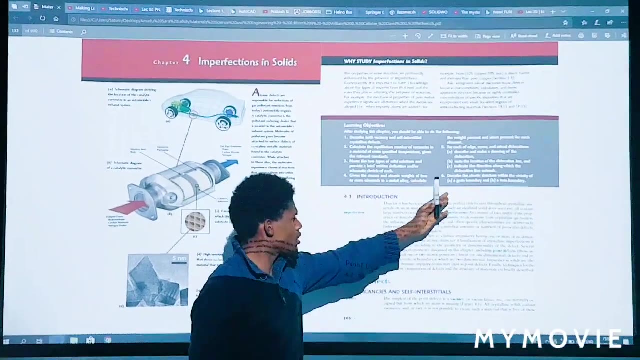 have another take away will be defects. we have edge and screw defect, so you should able to calculate these things and mix the effect. so only then you can able to understand these imperfections and then try to control these imperfections and we're going to talk about. 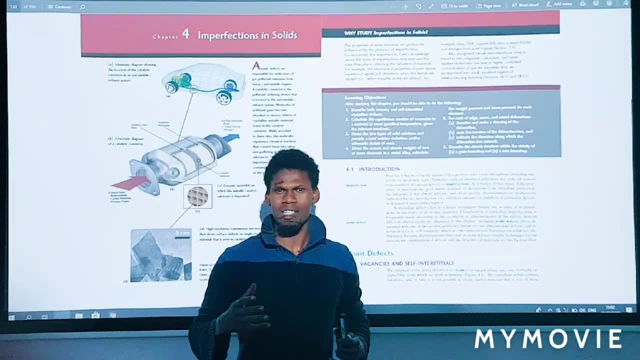 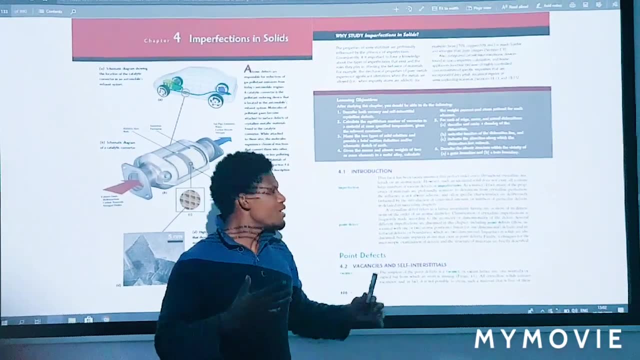 great boundary and twin boundaries. these are very, very important things because we know as human beings, we have what we call twins right. this is the same thing that is happening in materials, so this will even help you some kind of analogies to understand what is happening. now we're going. 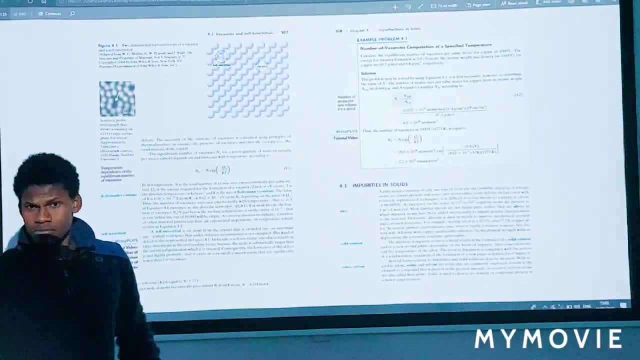 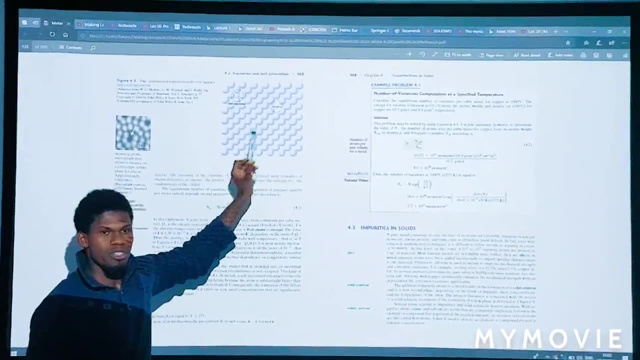 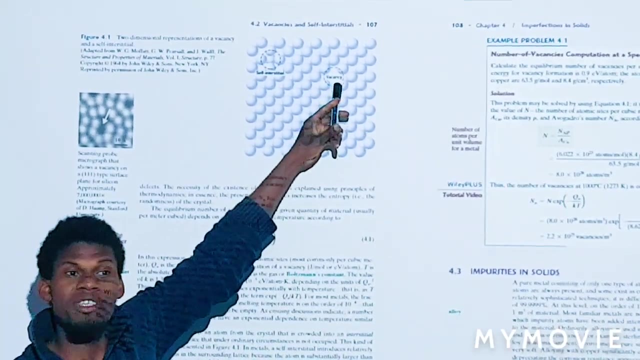 we start with vacancies. here is a typical example of vacancy and interstitial. a vacancy is, if you see, we look at the atoms, the atoms are arranged in a period, but however, if you look at this point here, an atom is missing here. so when an atom is missing, we say there is a vacancy. 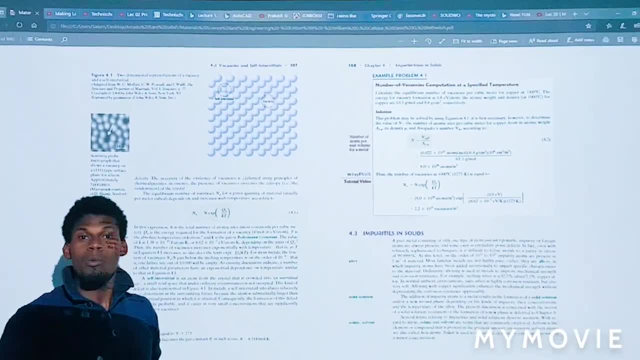 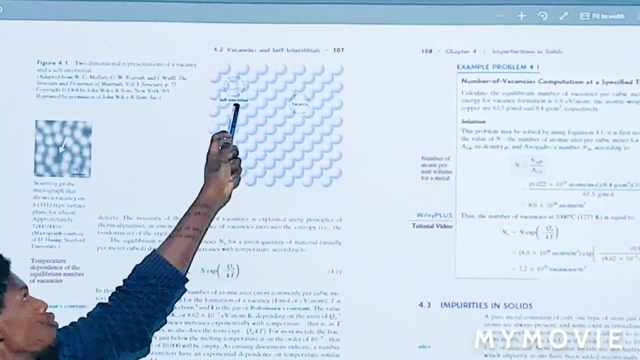 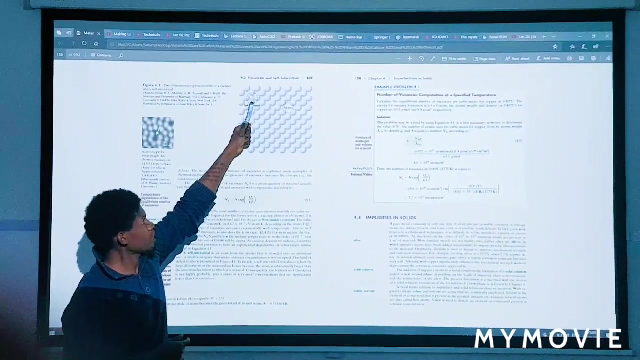 and in some cases, these atoms, you can find them somewhere else. if you look at here, there is an atom here, here the atom does supposed to be here, so there, this we call cell interstitial. and why we call the cell interstitial? because this atom that is here is the same as this, for 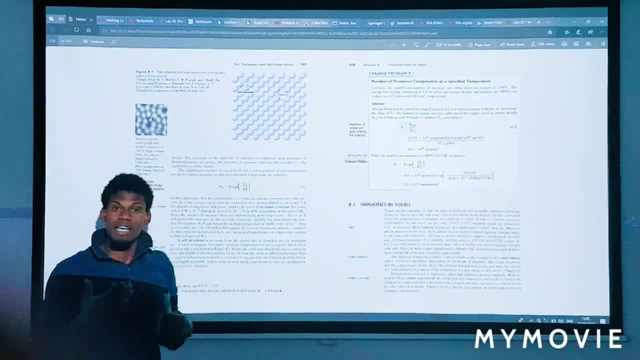 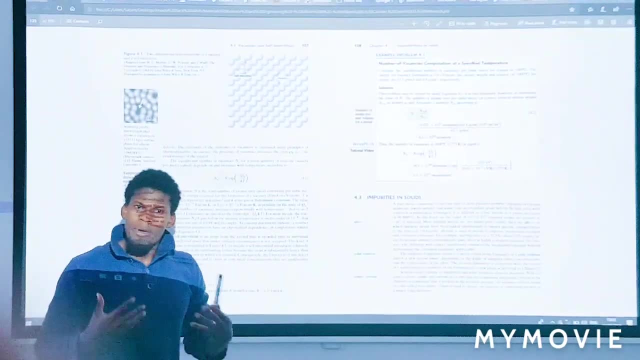 the atoms. but here there is no atom. we are not supposed to be an atom. so we say these are vacancies, and within a material we should able to calculate how many of these vacancies are here. so how can we do that? first we needed to come up with some mathematical equations to do. 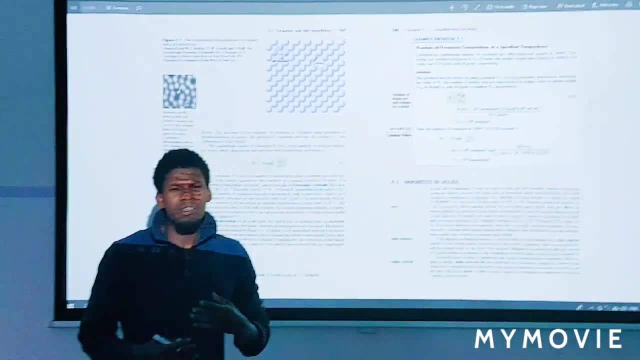 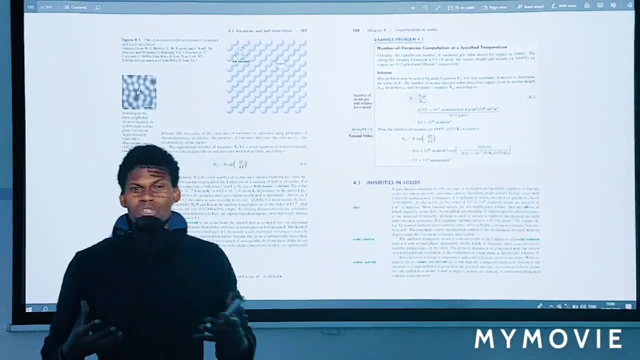 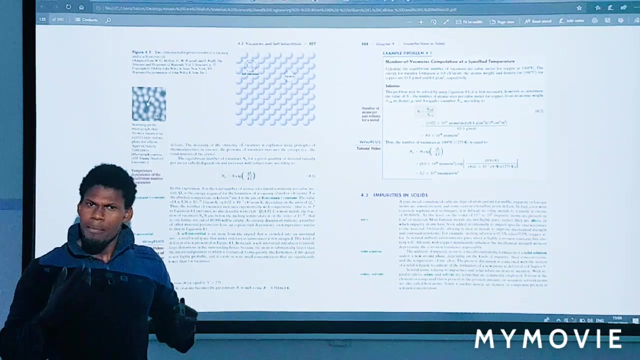 that to calculate the number of vacancies- and this, we need to have little knowledge of thermodynamics and the principles of thermodynamics- is just the measure of entropy, and entropy is just randomness, how things occur. randomly, because now, with this vacancy, what happened is that, because the atoms are vibrating, the atoms will try to occupy this space. and when? 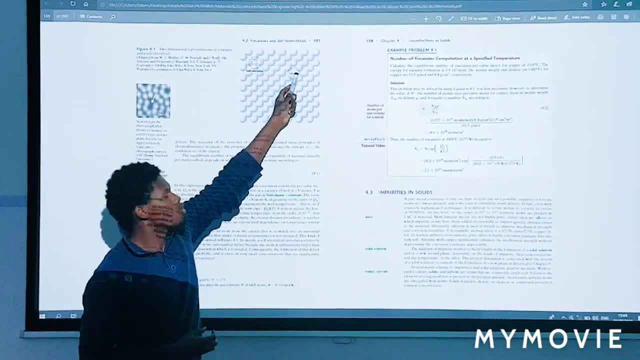 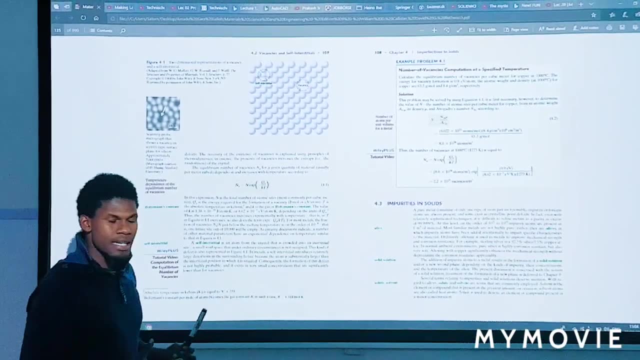 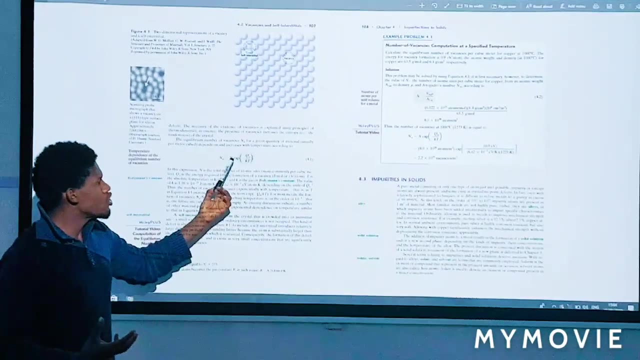 an atom come here, the vacancy will move over here in the next atom. so we can calculate these vacancies. so that way we come up with this formula mathematically. and this is a very simple formula to calculate the number of vacancy within a material all you need to have is the number. 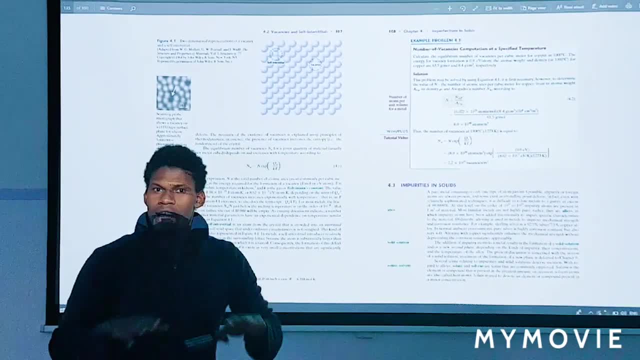 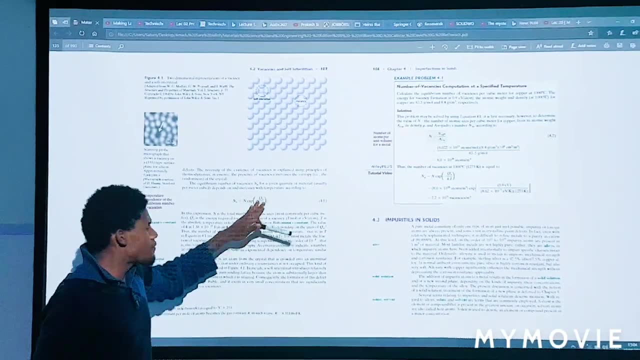 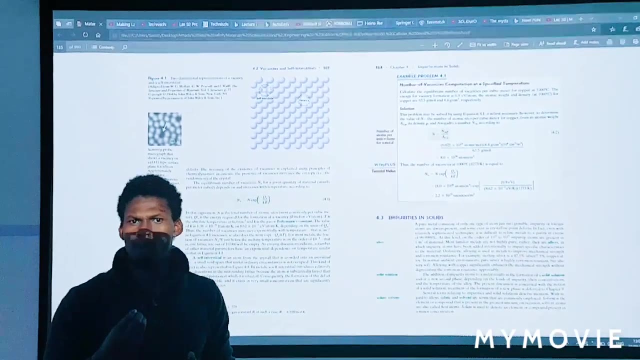 of interstitial site under normal conditions, if we assume that the material is perfect, how many lattice side this material have? and then you have the exponential value of qv over kt. qv is just the energy that is required to remove one atom within the lattice side, because we this is measured with electro volt and k. there is the boltzmann constant, which 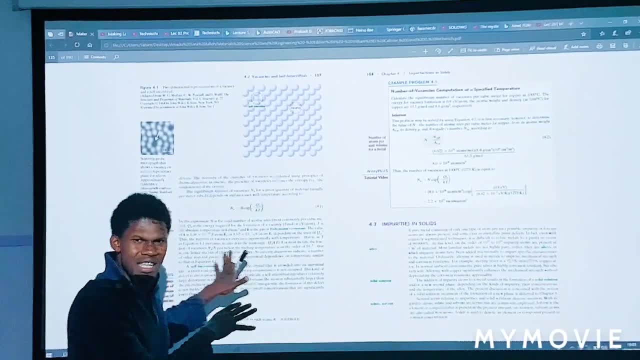 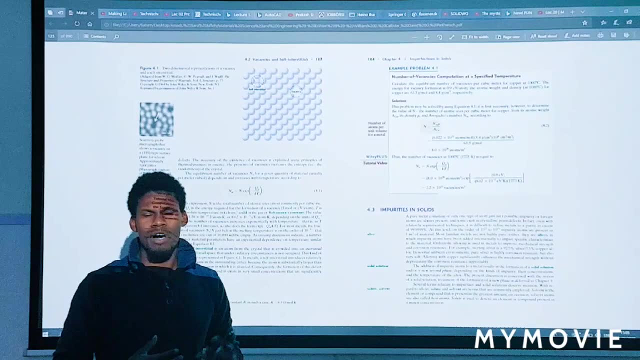 we can talk about. but the purpose of this is not just to memorize these things, but rather to able to to come up with these things. it's assuming you are individual of the forest, you are, you happen to have copper and zinc, so you should able to come up with these calculations, to calculate how many. 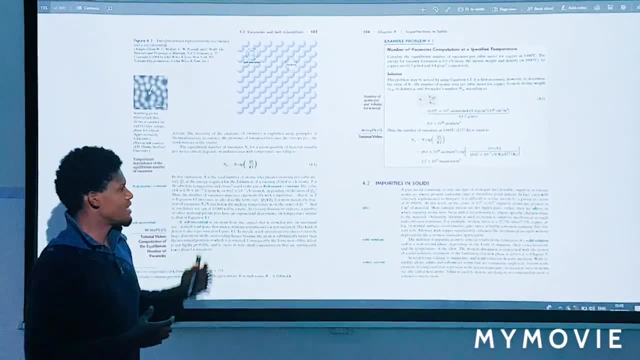 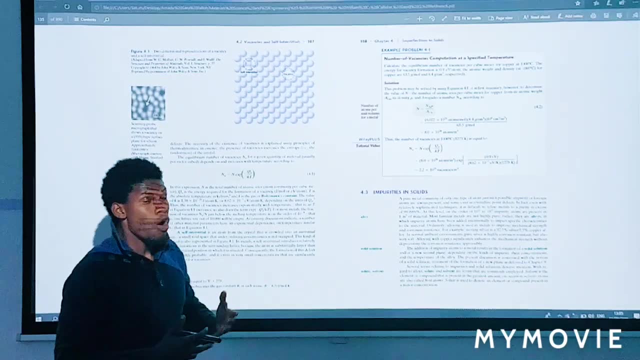 percent of copper, how many of zinc is there and how many vacancies are available. so that's exactly what we are doing here: we are calculating the number of vacancies that are available. in this we are calculating the equilibrium number of vacancies of copper, and, of course, the temperature is very, very important. at what temperature? because we know that when the 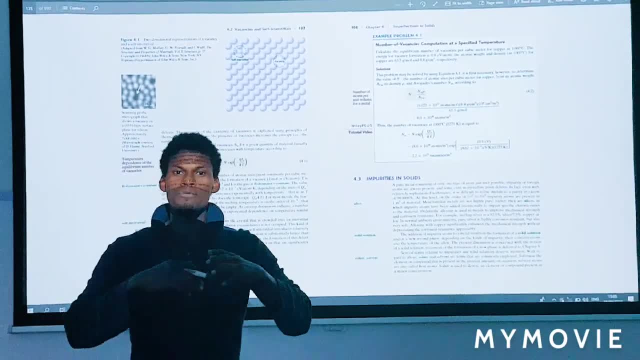 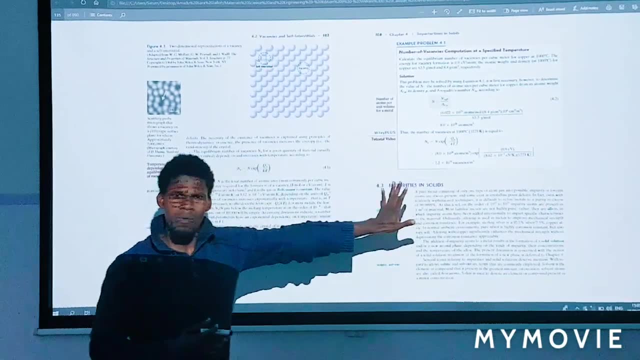 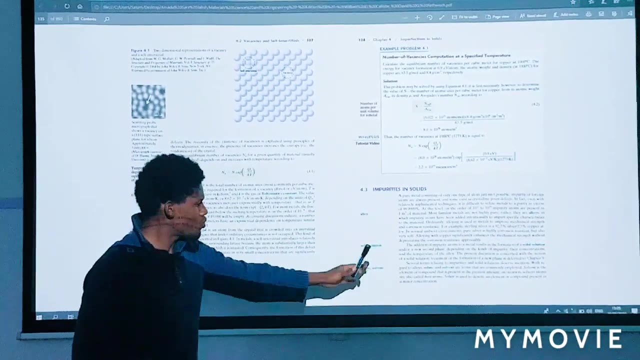 temperatures are higher. you should know that. then we have randomness, we have some higher degree of randomness. so this is the mathematics. but we are not going to worry ourselves today for these mathematics. we just want to understand the basic concept of imperfections and solids, and we talk about solid solutions solvent when we have 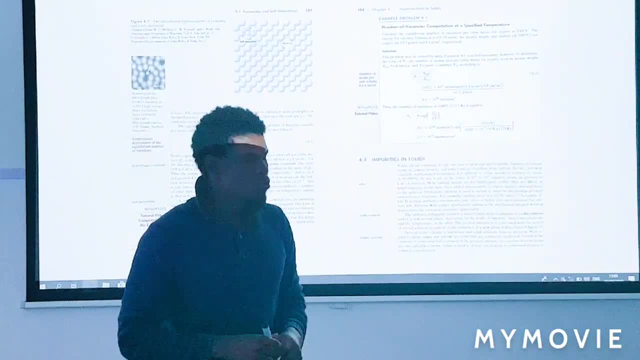 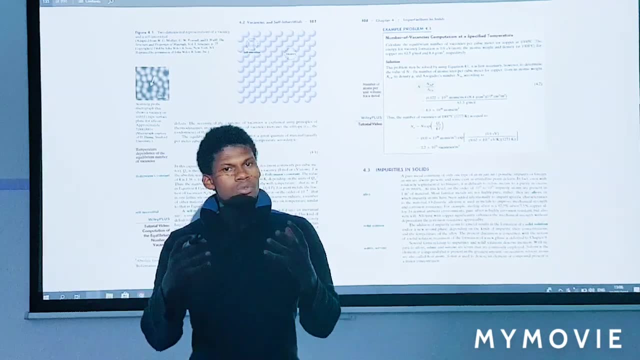 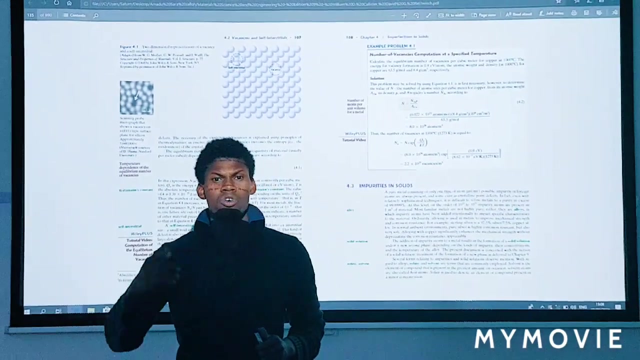 I said earlier on zinc and copper, you should able to know which one is the solid and which one is the solvent and, for example, if we have a complete material that is a copper, let's say, for example, 100, or let's say 99.999, because you you can never have a material that is 100. 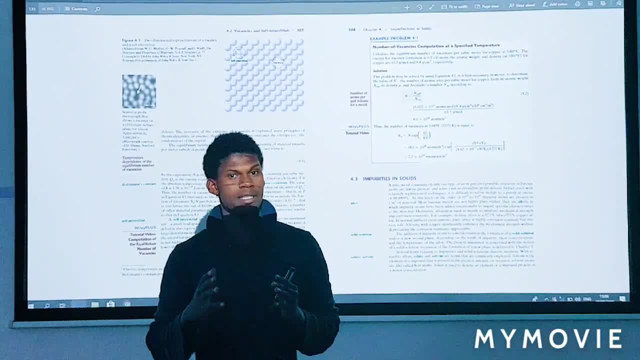 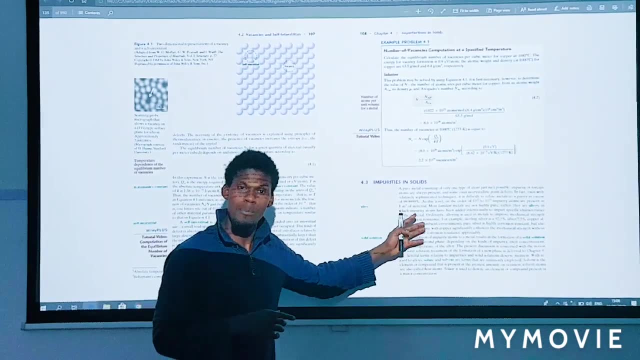 you can have material that is for decimal places, percentage, as this is how far we have tried. but you can maybe help you in some way or another because we might go into more and more detail. but you can maybe help with some sophisticated technologies to have more pure material. but pure materials are 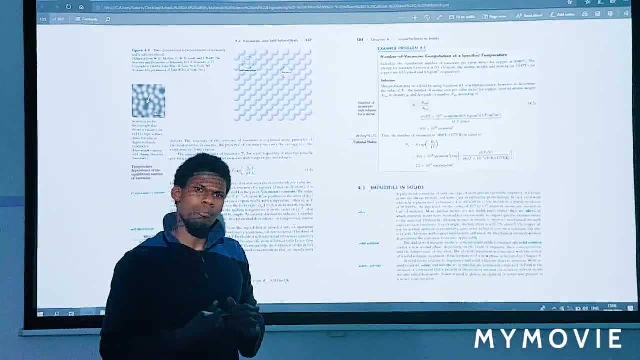 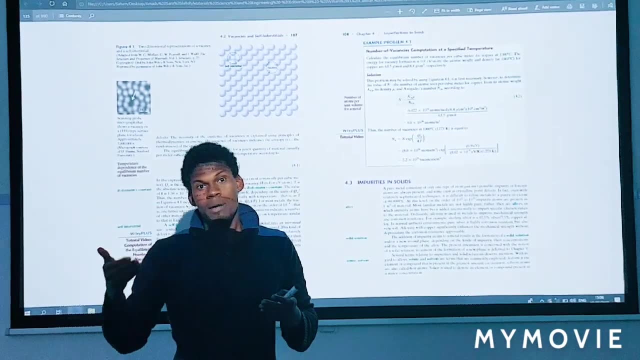 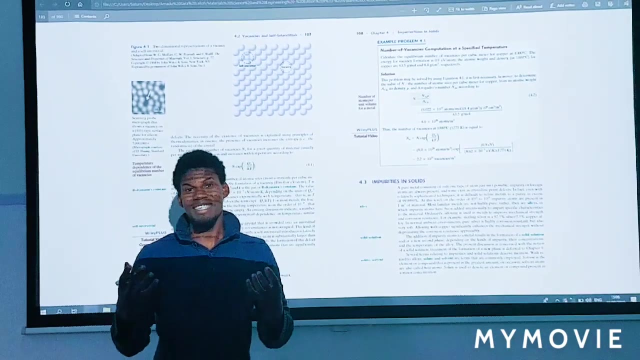 always soft. so if we want to enhance the mechanical properties, we need to deliberately put some other atoms of other material impurities within this material. and then we take zinc. so if we have 70 copper and 30 zinc, what will happen? that this material become much stronger, comparing. 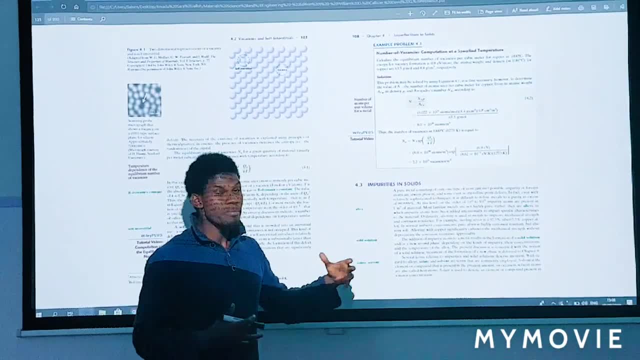 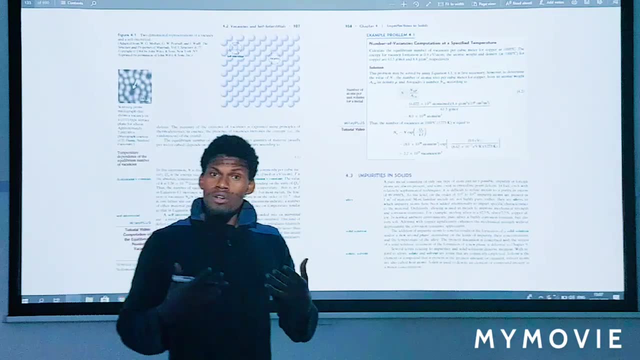 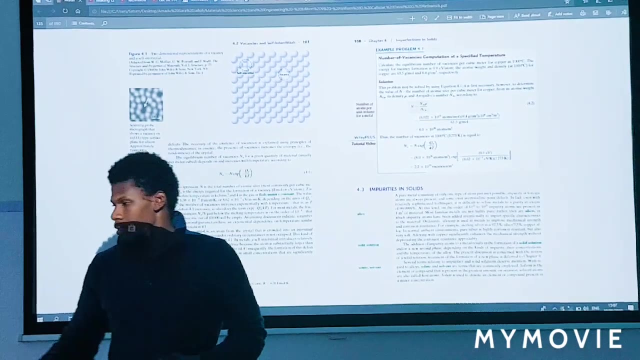 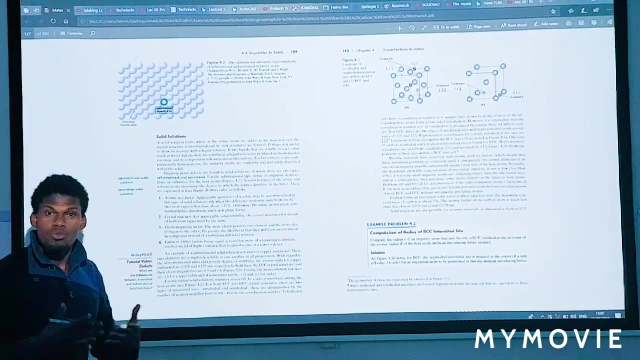 pure copper. so copper is weaker, so, and this will make the material become more stronger, and so copper here will be the, the solid, and then solvent. there will be zinc, and this we call grass today, which is 70 copper and 30 percent zinc. and we have, we have- some rules. if there is no rules, there is nothing that exists. we should. 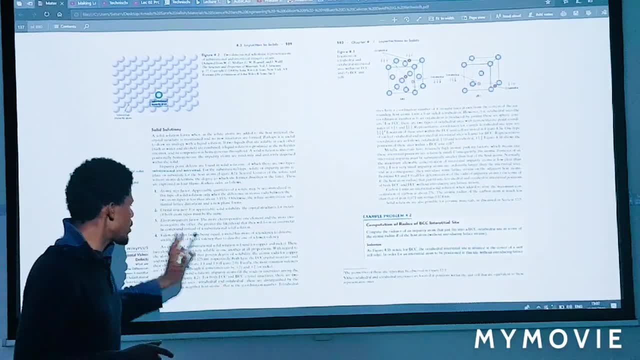 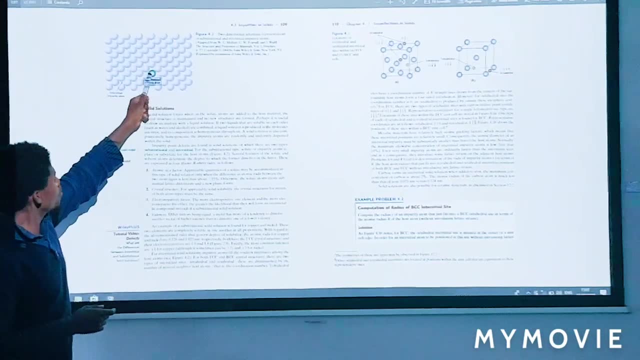 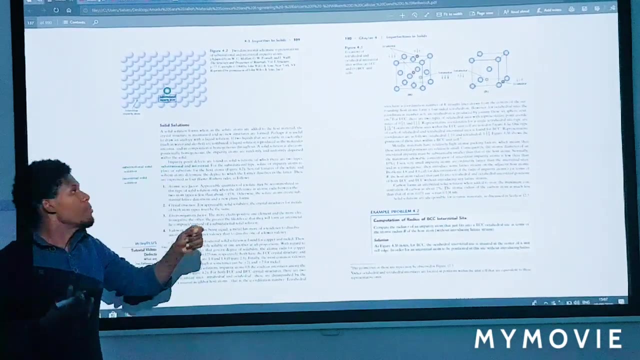 have roots, and exactly, in material science and engineering. we also have some rules. we talk about atomic size factor, how size the atom is. so suppose, in here you see this atom is green but the other ones are blue. but this can substitute for this, for the atoms. why? because the atoms, the sizes are the same. 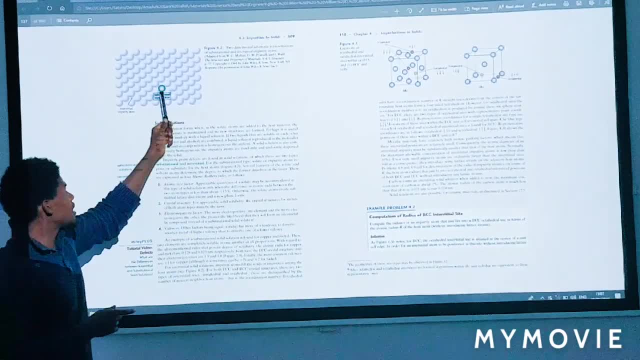 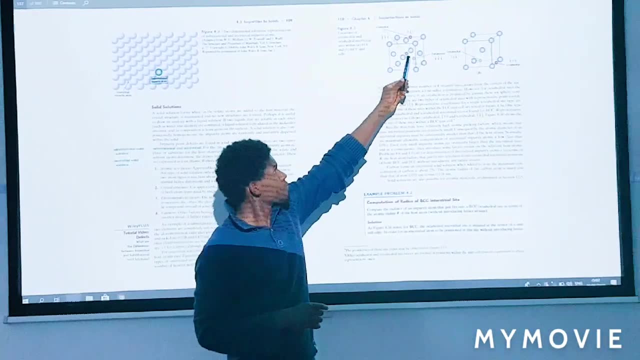 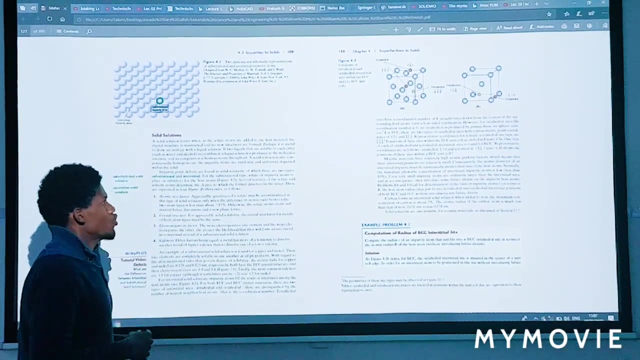 this is what we call this substitutional solid solution, because the size of the atom is the same. but when the size of the atoms are different, for instance here you can see- these are much bigger. so this we call interstitial solid solutions. so atoms are occupying an interstitial position. 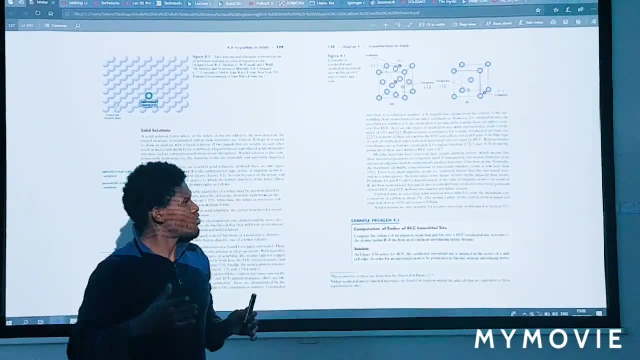 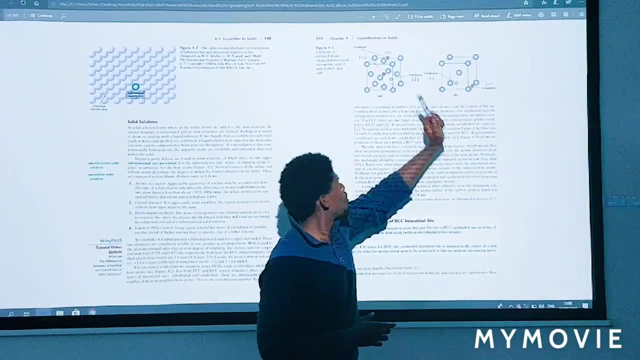 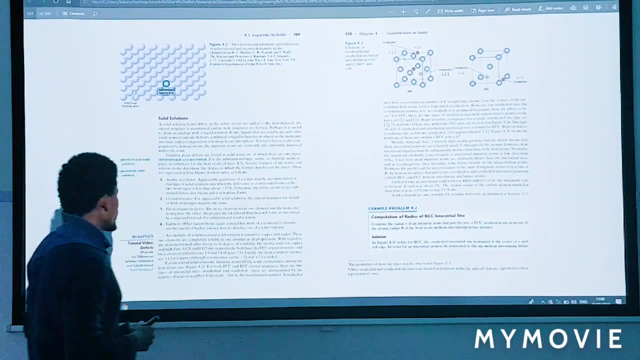 remember, when we talk about the fcc, bcc crystal structure, we talk about that and this is the fcc crystal structure. look at where the atoms are residing at the corners and when atoms reside here. this is fcc. we say these are octahedral and these are tetrahedrals and then decrease structure.